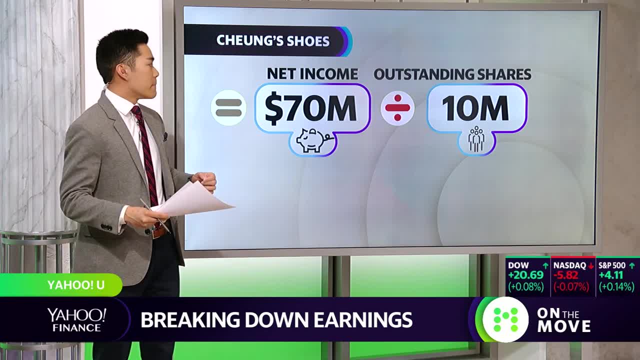 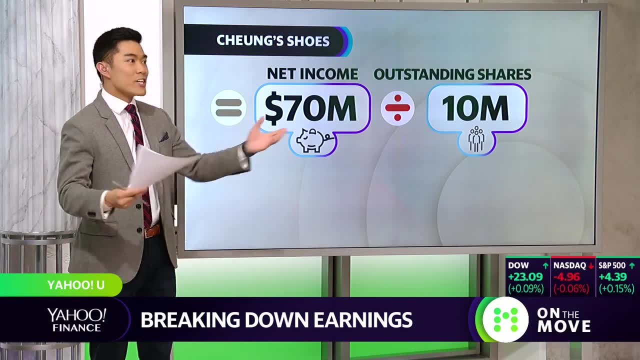 that's how much I have after I account for all of those changes. But now we're looking at how much money do I give out to the shareholders who have stock in Chung's Shoes. So, Julie and Adam, you have shares in Chung's Shoes, So you are part of the 10 million. 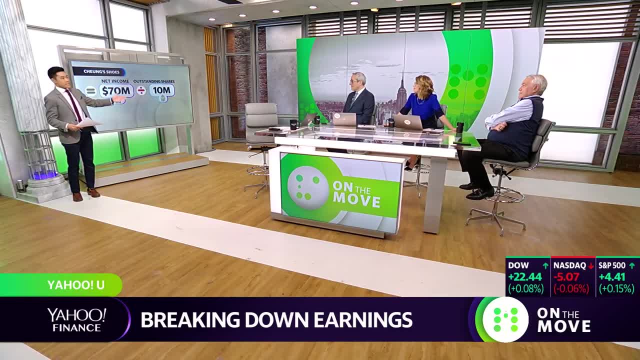 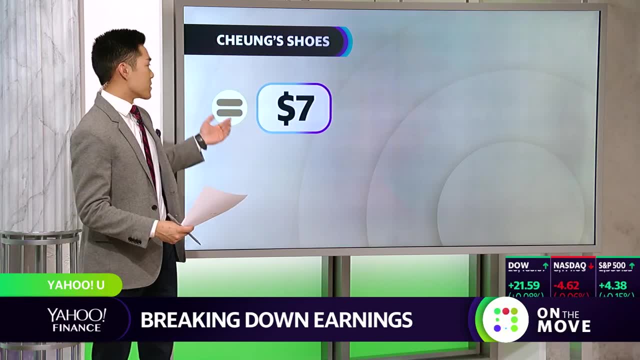 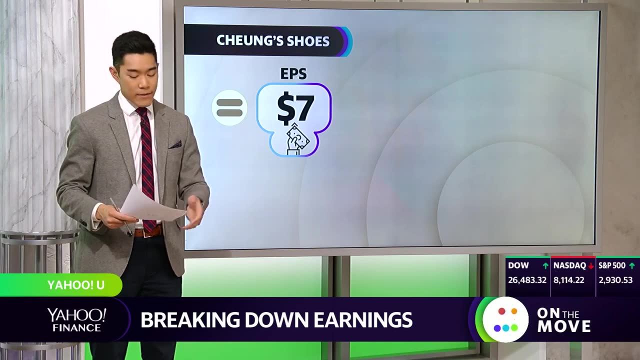 outstanding shares that exist. So we divide 70 million by 10 million, That gives us the earnings per share And EPS is basically the bottom line. That is effectively $7 when we divide 70 by 10.. And that is how much money each share will get in terms of the amount of earnings that I have made. 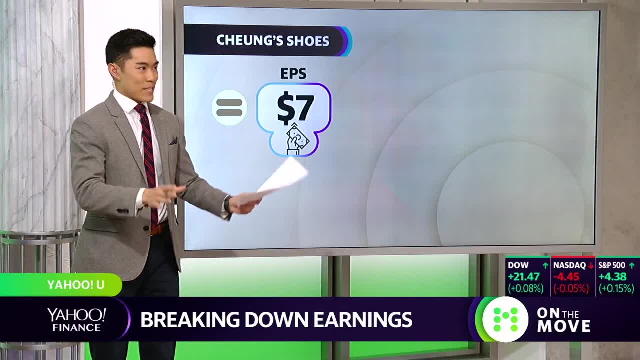 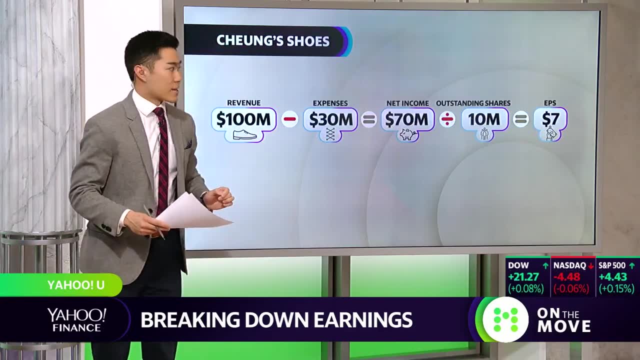 Now, this is a very simplistic way of looking at it. This is basically in its purest form. It gets a little bit more complicated than that. This is the whole equation. So again, top line revenue, bottom line being net income, EPS being what we 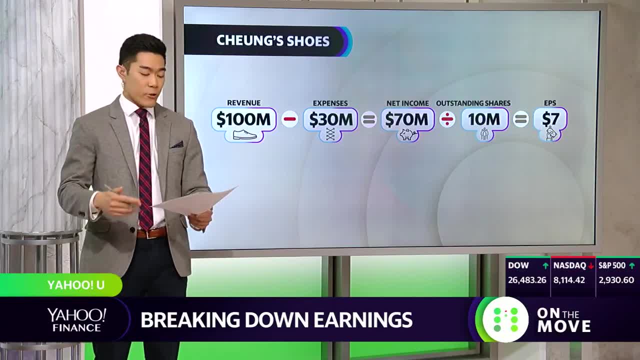 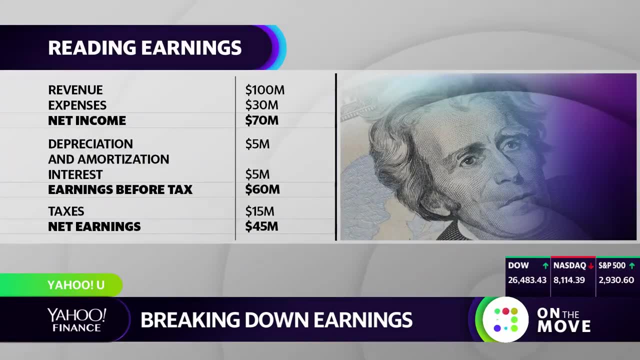 talk about in these earnings reports, But actually, in reality, there's a lot more other income lines that are on the income statement as well. We talk about EBITDA, for example. right, What does EBITDA mean? Well, EBITDA is an acronym. It stands for earnings before interest taxes: depreciation. 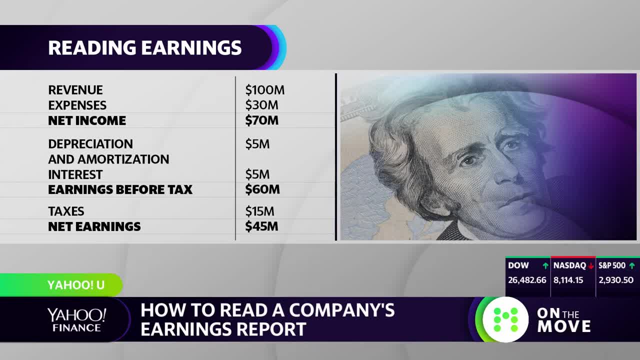 and amortization. So in reality, you'll see on the screen ahead of you that there's, in addition to net income, you have to pay for depreciation. If I have a warehouse, for example, that loses value over time, or equipment that also loses value over time, you also have 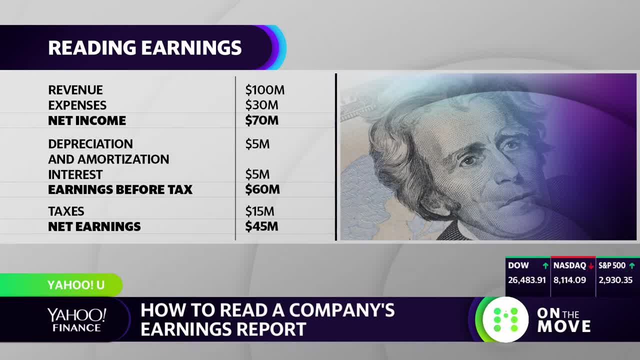 interest that you have to pay because I had to take a bank loan to get the mortgage on that warehouse or buy that equipment. And of course, you can't forget about taxes, what I owe to the state, what I also owe to the federal government. So on the bottom line it's really the net earnings. 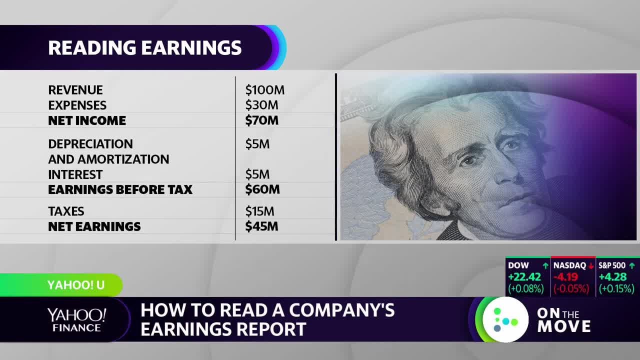 of $45 million. in this fake scenario, Of course, EBITDA is basically controlling. for all those things, It's really out of my control. I don't control the tax rate, I don't control how much my warehouse depreciates. So when we talk about EBITDA, in this case it would be $70 million. 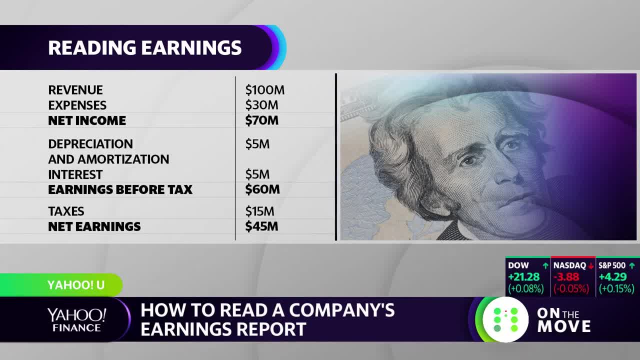 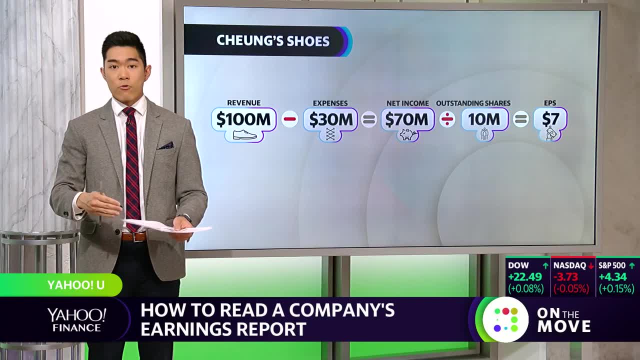 That's simply the $100 million that I made, subtracted by the $30 million that I had to spend to make those goods. Now we talk also about an earnings recession. That's something we've been hearing a lot about recently. The earnings recession is kind of talking about. 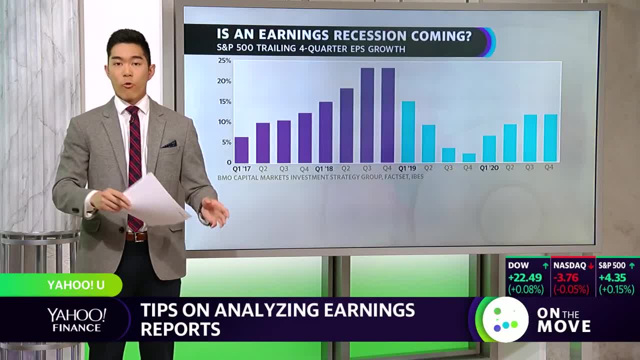 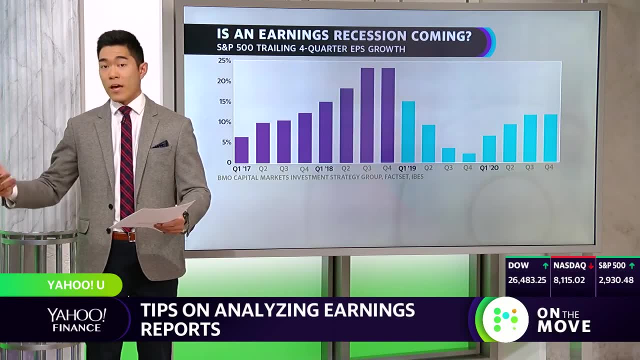 guidance, for example. So we've heard a number of companies over the fourth quarter, and also in the first quarter, talk about how they actually have a gloomier outlook for 2019.. Partially because of an economic slowdown abroad that might spill over into the US.